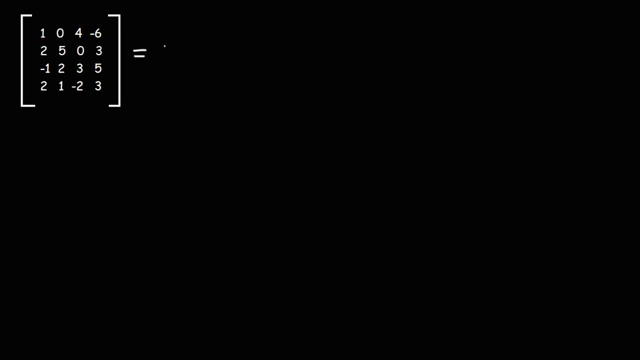 So let's start with the first one. The first coefficient is 1, and it's located in row 1,, column 1.. So we're going to eliminate row 1 and column 1. And what's left over are the numbers that we need for the 3x3 matrix that we're about to write. 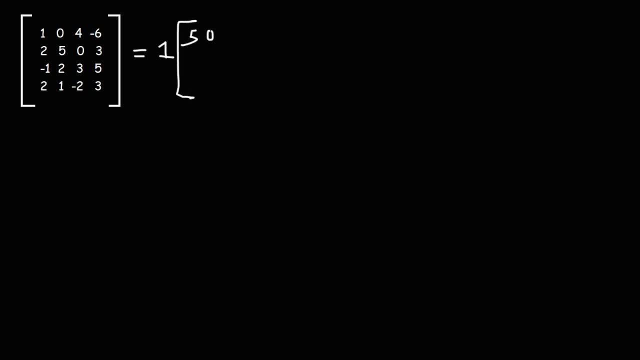 And so that was 5, 0, 3, 2, 3, 5, 1, negative: 2, 3.. Now let's move on to the second number in the first row. Notice that we have a positive one here. 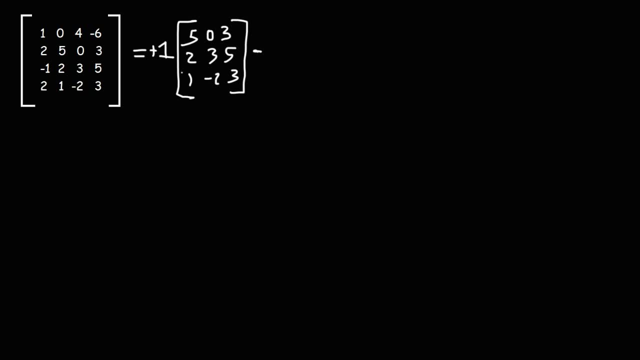 The next one is going to be minus. The signs will alternate, So minus the next number, which is 0.. And then we're going to write the next 3x3 matrix. So 0 is in row 1, column 2.. 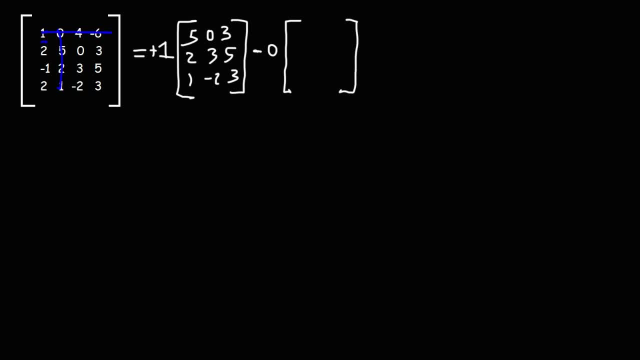 So the numbers that we have: 2, negative 1, 2, and then 0,, 3,, 3,, 5, negative 2, 3.. We're going to put that in the next 3x3 matrix. 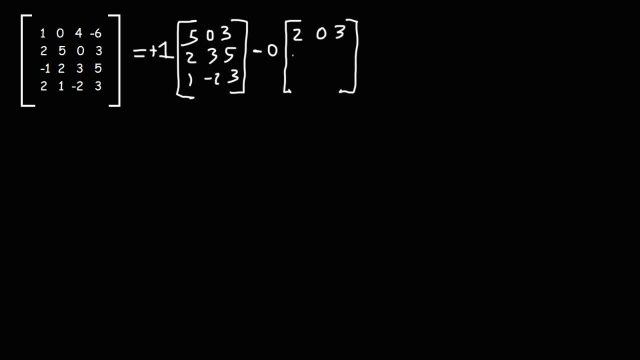 So that was 2, 0, 3.. Whoops, Negative: 1, 3, 5.. 2, negative: 1, 3, 5.. 2, negative: 2, 3.. So just to review: the 0 was in row 1,, column 1.. 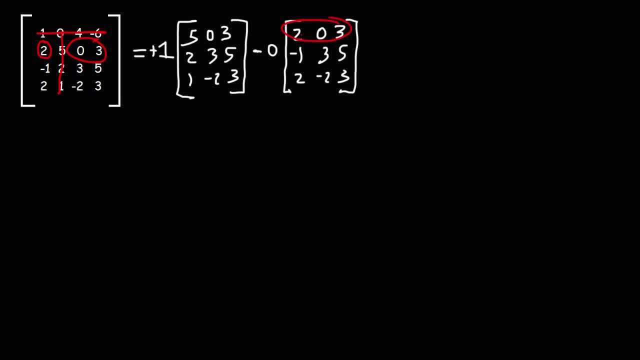 And you can see the numbers here: 2, 0, 3.. That's in the second row. In the third row we have negative 1, 3, 5.. And then in the last row we have 2, negative 2, 3.. 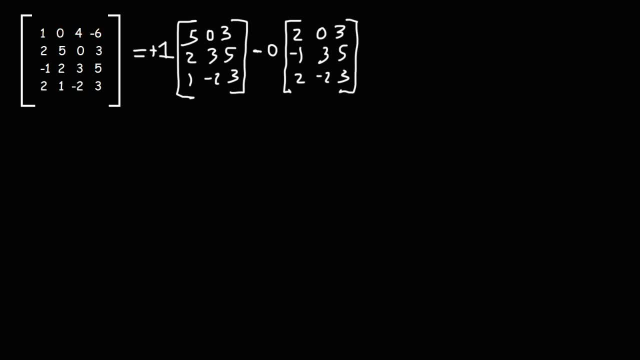 Now let's move on to the next number in row 1.. So that's going to be 4.. And it's going to be positive 4, because the previous coefficient was negative. So 4 is in row 1, column 3.. 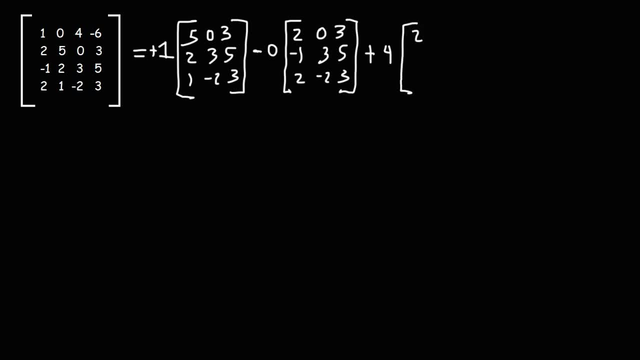 And so that's going to leave behind the numbers 2, 5, 3,, negative 1, 2, 5, and then 2, 1, 3.. I'm taking this one step at a time, so you can follow along. 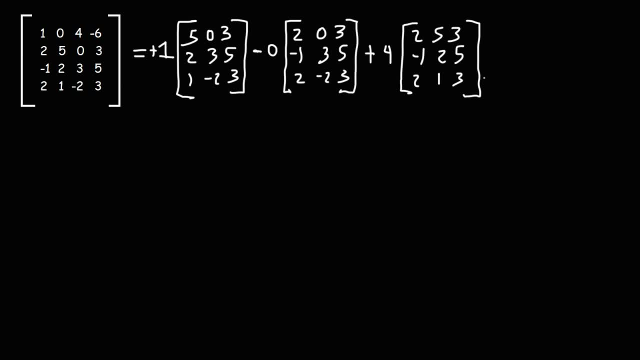 Now we're going to move on to the last number In the first row. Now the sign is going to change from positive to negative, So it's going to be negative, And then the number that we see here Minus 6.. 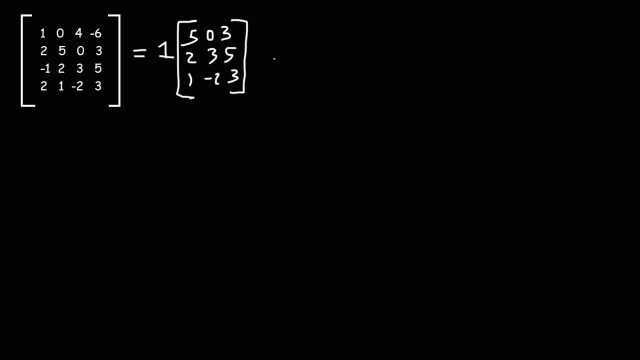 Now let's move on to the second number in the first row. Notice that we have a positive one here. The next one is going to be minus. The signs will alternate. So minus the next number, which is 0. And then we're going to write the next 3x3 matrix. So 0 is in row 1, column 2. So the numbers that we have, 2, negative 1, 2, and then 0, 3, 3, 5, negative 2, 3. 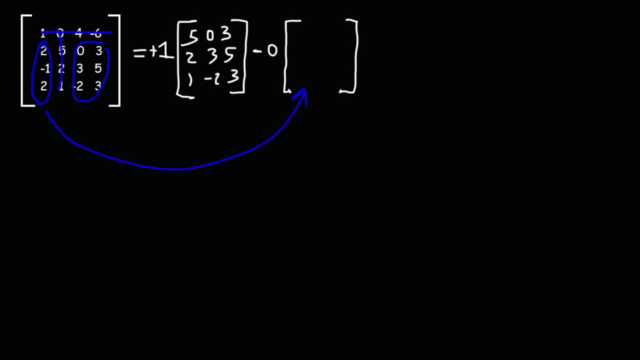 We're going to put that in the next 3x3 matrix. So that was 2, 0, 3. Whoops. Negative 1, 3, 5. 2. 2, negative 2, 3. 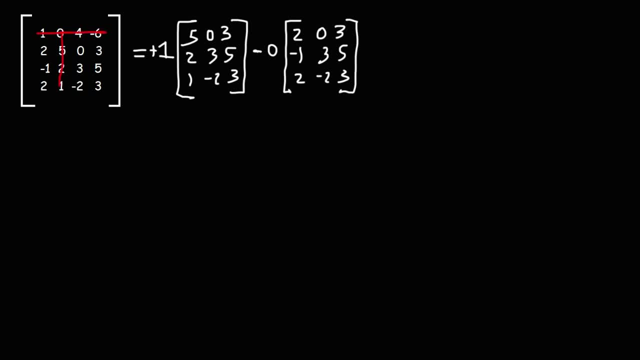 So just to review, the 0 was in row 1, column 1. And you can see the numbers here. 2, 0, 3. That's in the second row. 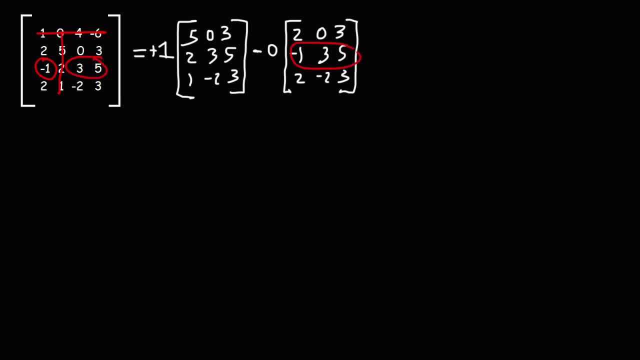 In the third row, we have negative 1, 3, 5. And then in the last row, we have 2, negative 2, 3. 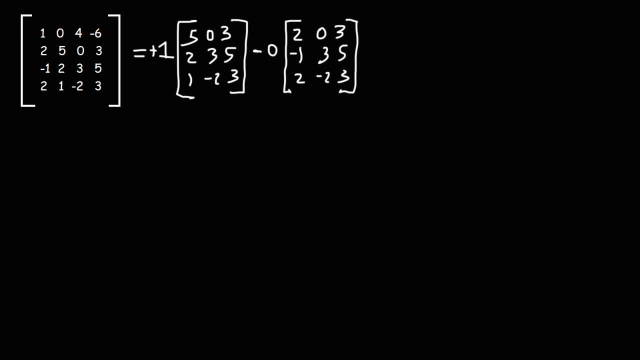 Now let's move on to the next number in row 1. So that's going to be 4. And it's going to be positive 4 because the previous coefficient was negative. So 4 is in row 1, column 3. 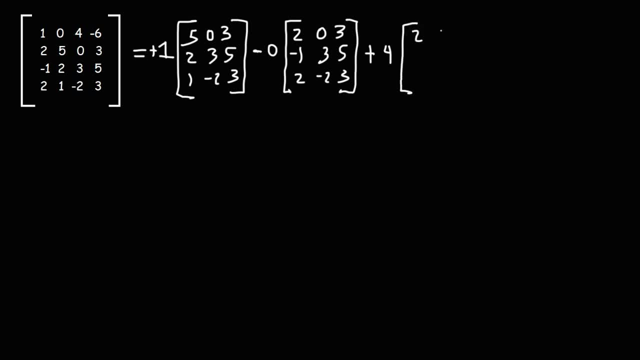 And so that's going to leave behind the numbers 2, 5, 3, negative 1, 2, 5, and then 2, 1, 3. I'm taking this one step at a time so you can follow along. Now we're going to move on to the last number. In the first row. 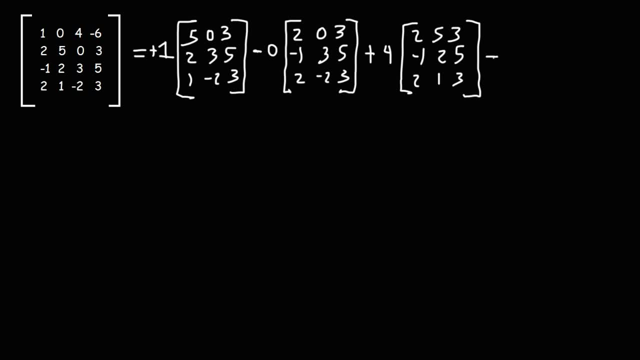 Now the sign is going to change from positive to negative. So it's going to be negative. And then the number that we see here. Minus 6. So negative 6 is in the first row, fourth column. 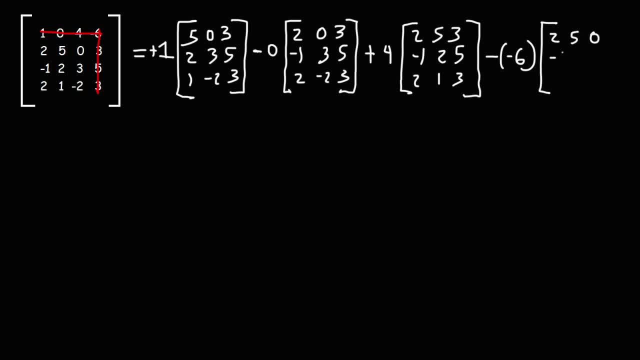 So we're left over with 2, 5, 0. Negative 1, 2, 3. 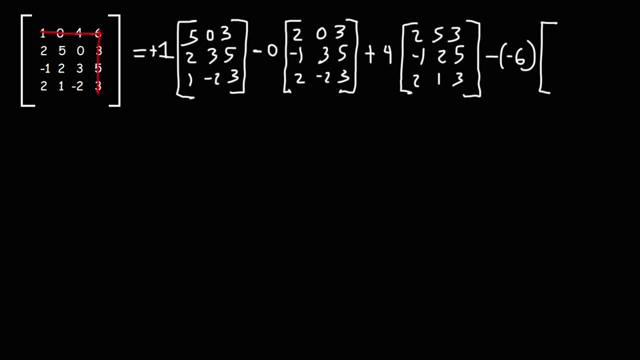 So negative 6 is in the first row, fourth column. So we're left over with 2, 5, 0.. Negative 1, 2, 3.. 2, 1, negative 2.. Now here's the reason. 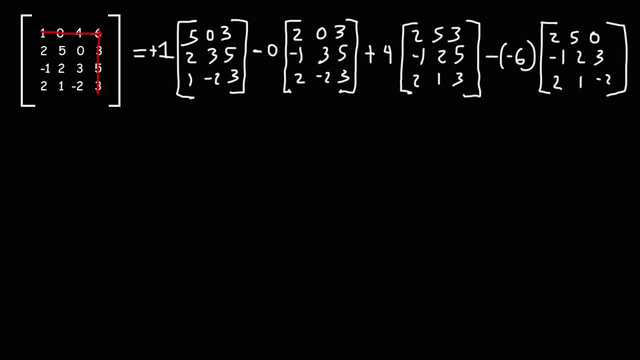 Why you want to identify the row or the column with the greatest number of zeros, Because 0 times this determinant is going to be 0. And thus this will simplify the work that you need to do, Because you need to find the determinant of each of these 3 by 3 matrices. 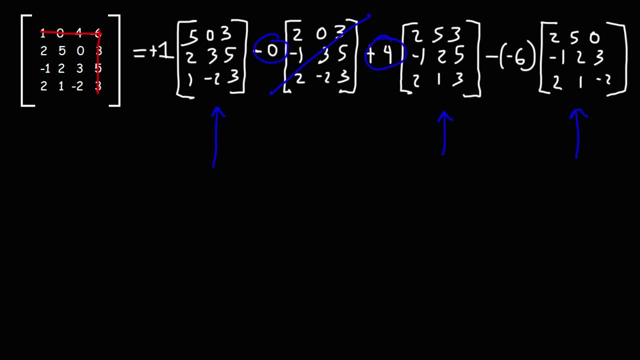 So the more zeros that you have, the less work that you'll have to do. Keep that in mind. Now let's evaluate the 3 by 3 matrices, One at a time. So let's start with the first one: 503, 235, 1, negative 2, 3.. 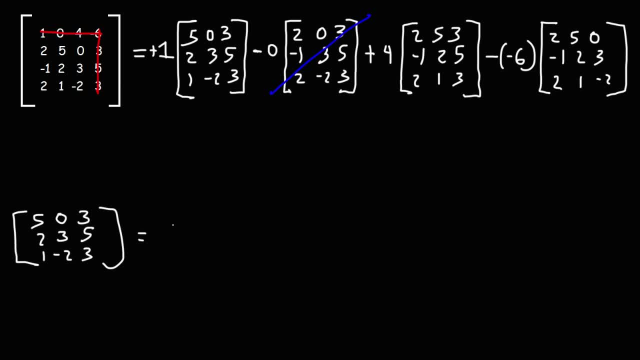 So let's use the first row. So we have 5 as the first number. If we take out row 1, column 1. We're left with a 2 by 2 matrix, And so that's going to be 3, 5, negative 2, 3.. 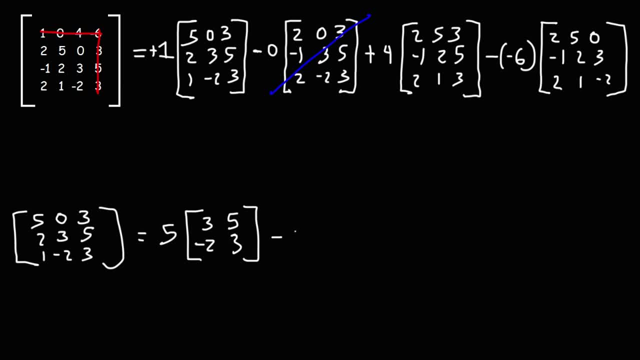 And then it's going to be minus. The next number is 0.. And 0 is in row 1,, column 2.. It leaves behind 2, 5,, 1,, 3.. And then plus the last number in the first row, which is 3.. 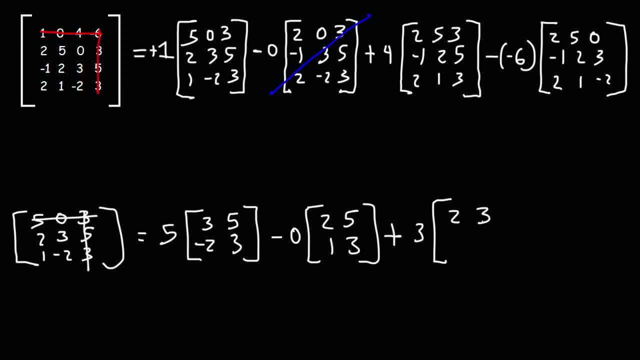 And that's in row 1,, column 3. Which leaves behind 2, 3, 1, negative 2.. Now to evaluate a 2 by 2 matrix, What you need to do is You need to multiply the first diagonal going in that direction. 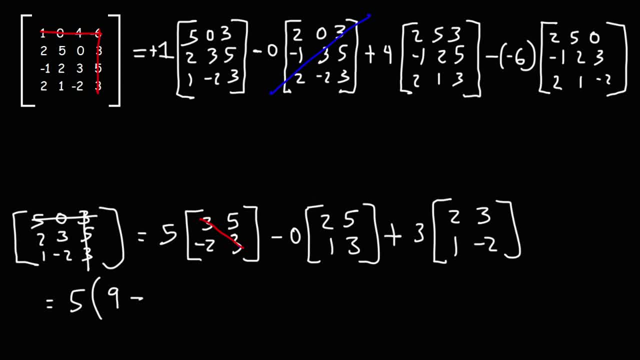 3 times 3 is 9.. And then minus the second diagonal going in that direction, Negative 2 times 5 is negative 10.. 0 times that determinant is 0. And then it's going to be plus 3.. 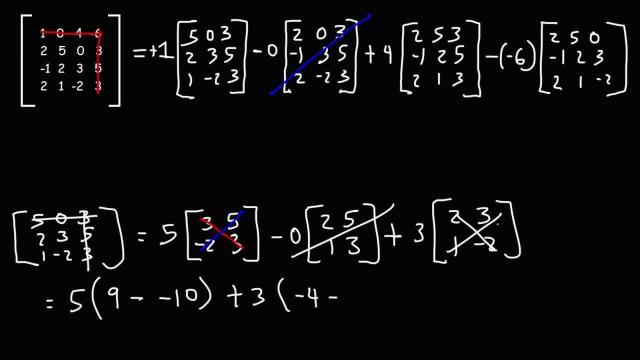 2 times negative, 2 is negative 4.. Minus 1 times 3,, which is positive 3.. So this is 9 plus 10,, which is 19.. And then 9.. Negative 4 minus 3 is negative 7.. 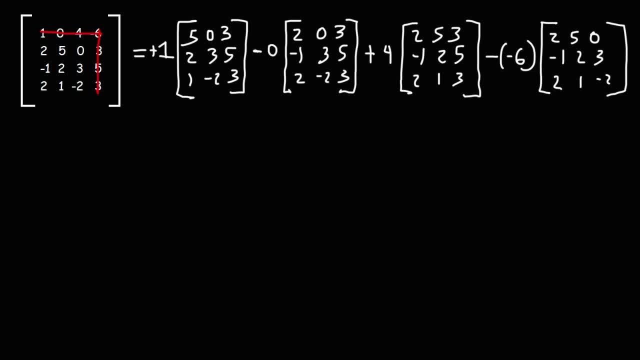 Now here's the reason. This is the reason why you want to identify the row or the column with the greatest number of zeros. Because 0 times this determinant is going to be 0. And thus, this will simplify the work that you need to do. Because you need to find the determinant of each of these 3 by 3 matrices. So the more zeros that you have, the less work that you'll have to do. Keep that in mind. Now let's evaluate the 3 by 3 matrix. 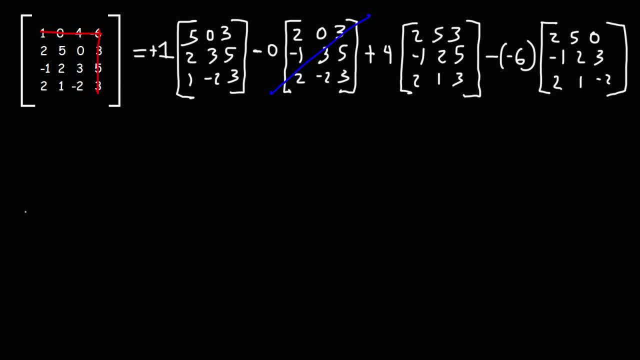 So let's start with the first one. 5, 0, 3. 2, 3, 5. 1, negative 2, 3. 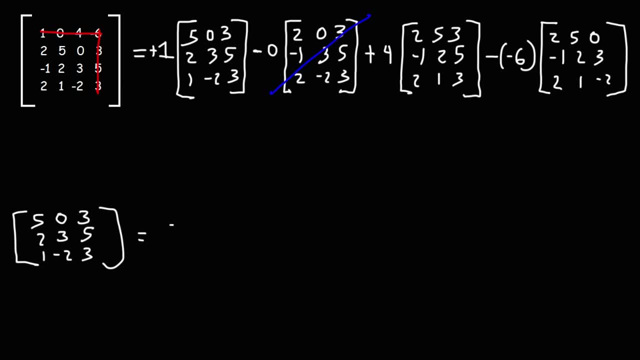 So let's use the first row. So we have 5 as the first number. If we take out row 1, column 1. We're left with a 2 by 2 matrix. And so that's going to be 3, 5, negative 2, 3. 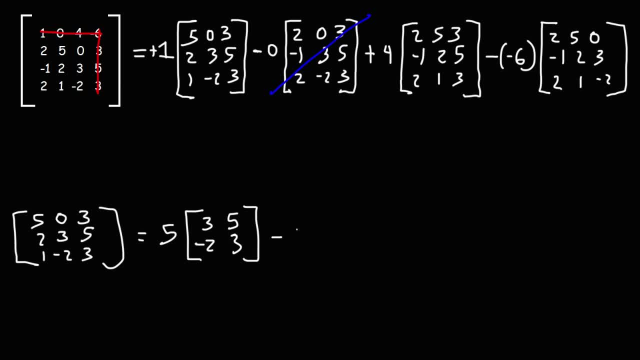 And then it's going to be minus. The next number is 0. And 0 is in row 1, column 2. It leaves behind 2, 5, 1, 3. 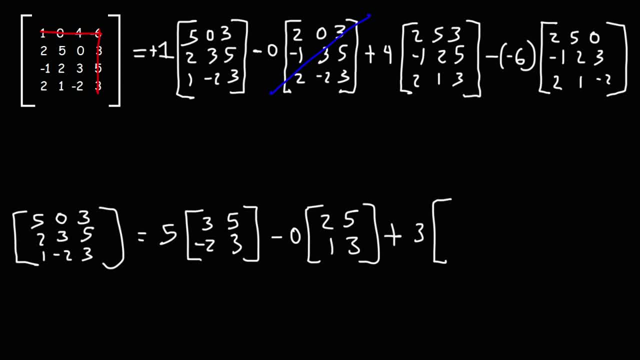 And then plus the last number in the first row, which is 3. And that's in row 1, column 3. 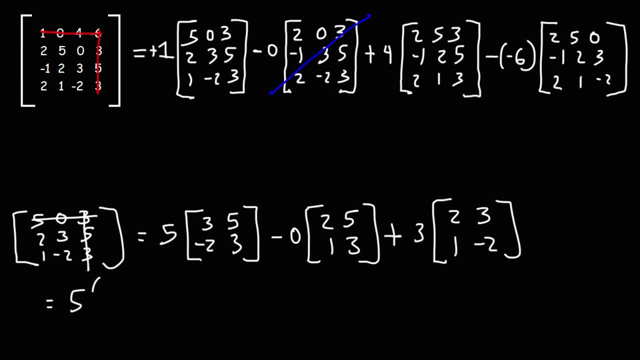 Now to evaluate a 2 by 2 matrix. What you need to do is, you need to multiply the first diagonal going in that direction. 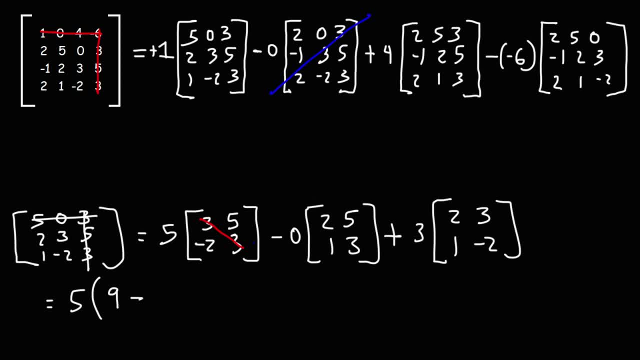 3 times 3 is 9. And then minus the second diagonal going in that direction. Negative 2 times 5 is negative 10. 0 times that determinant is 0. 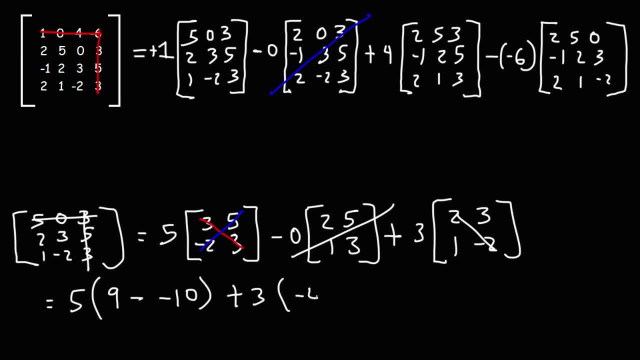 And then it's going to be plus 3. 2 times negative 2 is negative 4. Minus 1 times 3, which is positive 3. So this is 9 plus 10, which is 19. And then negative 4 minus 3 is negative 7. 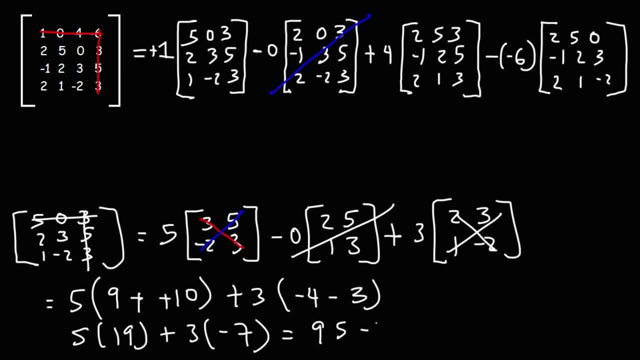 5 times 19 is 95. 3 times 7 is 21. 95 minus 21 is 74. 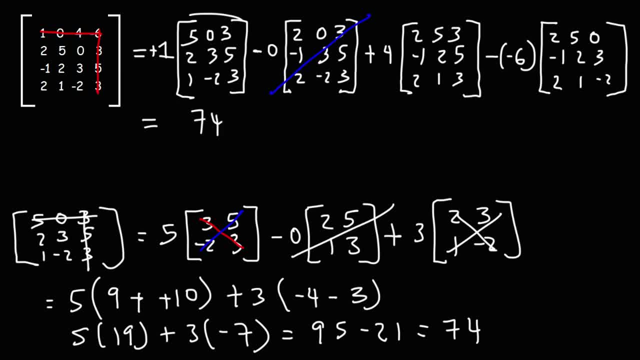 So that's the value, or the determinant rather, of this particular 3 by 3 matrix. So now let's repeat the process for the other two 3 by 3 matrices. 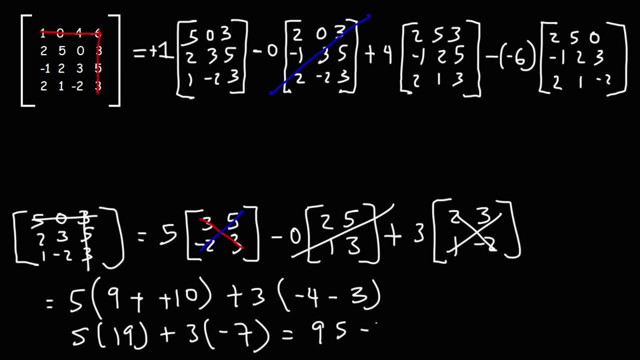 5 times 19 is 95.. 3 times 7 is 21.. 95 minus 21 is 74.. So that's the value, or the determinant rather, of this particular 3 by 3 matrix. So now let's repeat the process for the other two 3 by 3 matrices. 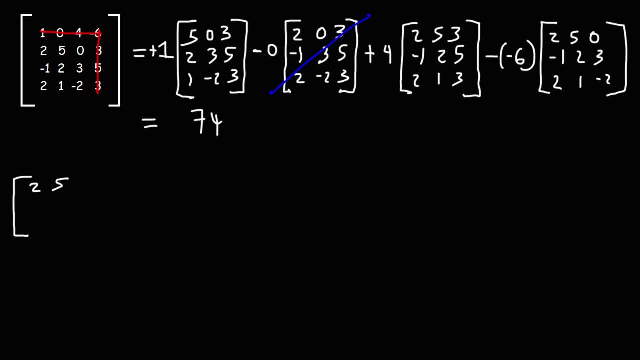 So let's move on to the next one: 2, 5, 3.. Negative: 1, 2, 5.. And then 2, 1, 3.. So let's use the first row again. We'll start with the first number, 2.. 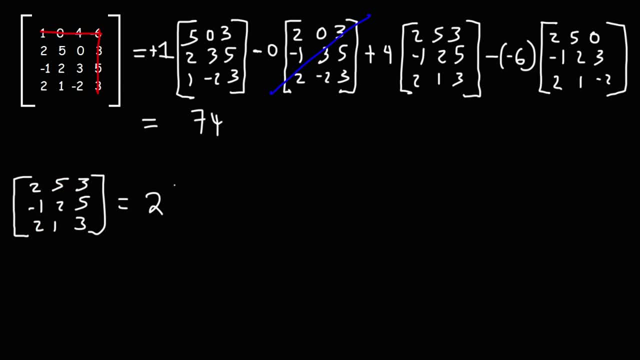 And it leaves behind 2, 5, 1, 3 in the 2 by 2 matrix, Then we need to alternate the sign. So we're going to use the second number, But we're going to put a negative sign in front of that. 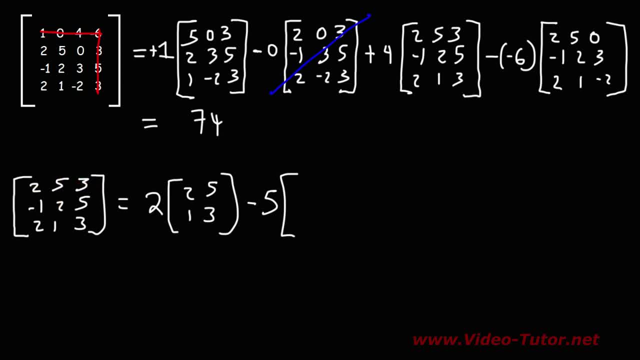 And we're going to have the numbers negative 1,, 5,, 2, 3.. Next, the last number in row 1 is 3.. And if we eliminate row 1,, column 3,, we're left over with negative 1,, 2,, 2, 1.. 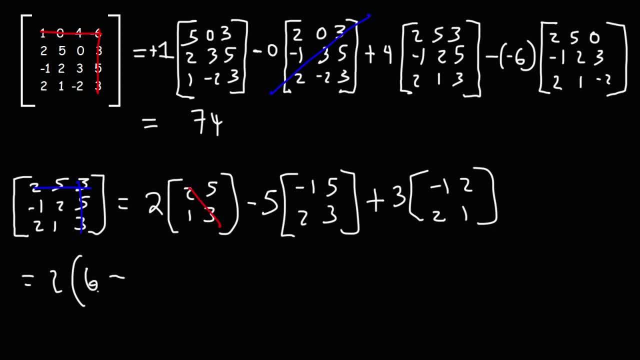 So we're going to have 2 times 3,, which is 6,, minus 1 times 5,, which is 5.. And then it's going to be minus 5.. And then we have negative 1 times 3.. 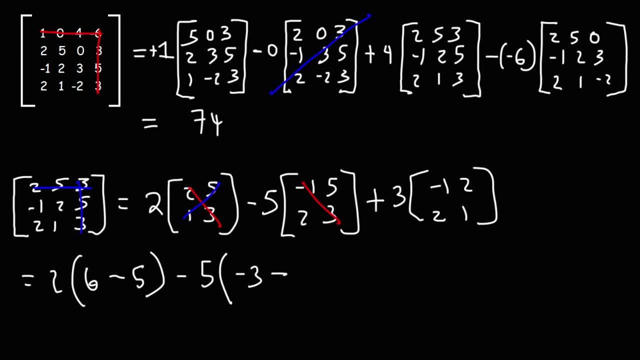 That is negative 3.. Minus, Minus 2 times 5,, which is positive 10. And the next negative 1 times 1, is negative 1.. And then minus 2 times 2,, which is 4.. 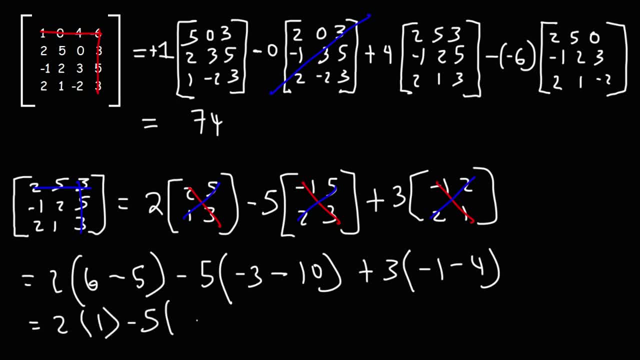 6 minus 5 is 1.. Negative 3 minus 10 is negative 13.. Negative 1 minus 4 is negative 5.. Negative 5 times negative 13.. That's positive 65.. 3 times negative: 5 is negative 15.. 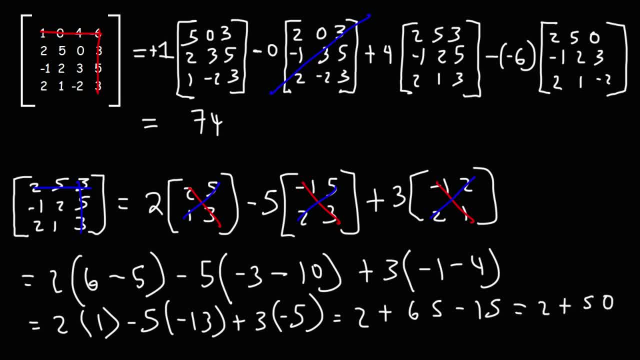 65 minus 15 is 50.. And 2 plus 50 is 52. So this is plus 4 times 52.. Don't forget the 4 here. And let's put a 0 for this particular 3 by 3 matrix. 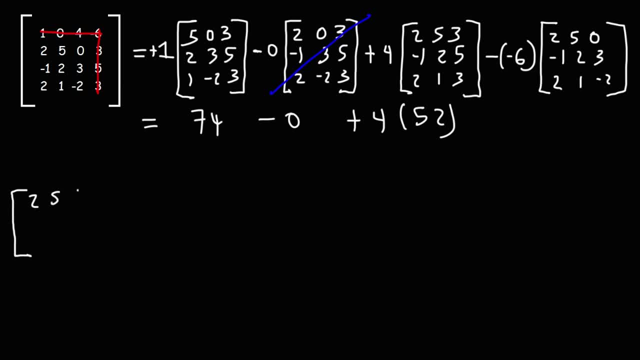 Now let's work on the last one. So the numbers are 2, 5, 0, negative 1, 2, 3, 2, 1, negative 2.. So, starting with the first number, 2.. 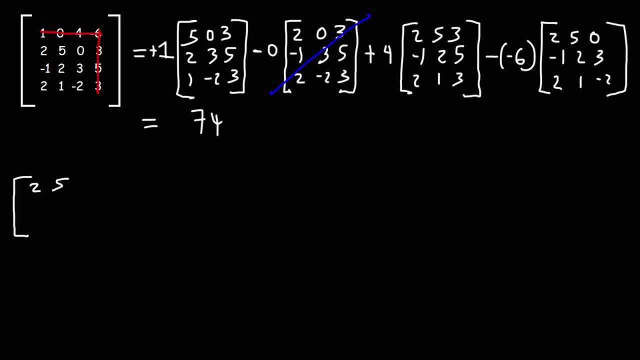 So let's move on to the next one. 2, 5, 3. Negative 1, 2, 5. And then 2, 1, 3. So let's use the first row again. We'll start with the first number 2. 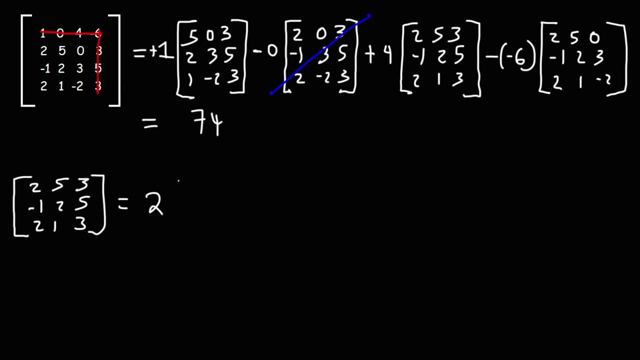 And it leaves behind 2, 5, 1, 3 in the 2 by 2 matrix. 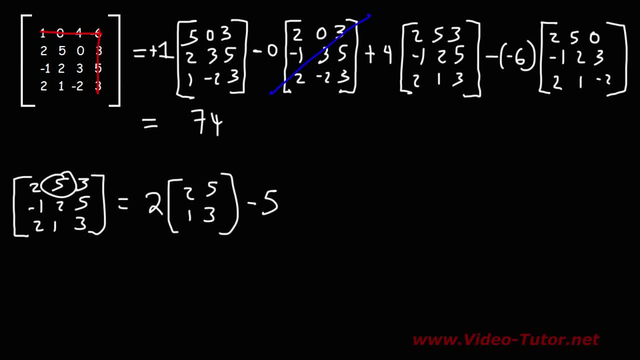 Then we need to alternate the sign. So we're going to use the second number, but we're going to put a negative sign in front of that. And we're going to have the numbers negative 1, 5, 2, 3. 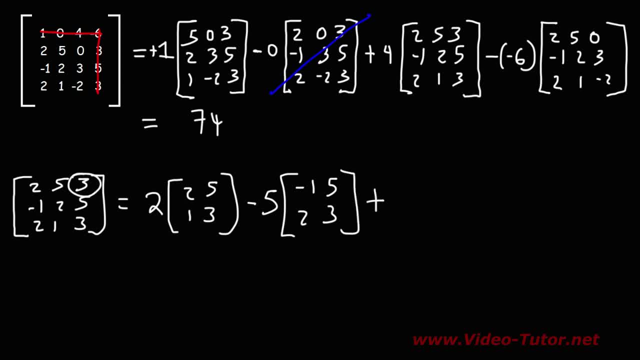 Next, the last number in row 1 is 3. And if we eliminate row 1, column 3, we're left over with negative 1, 2, 2, 1. 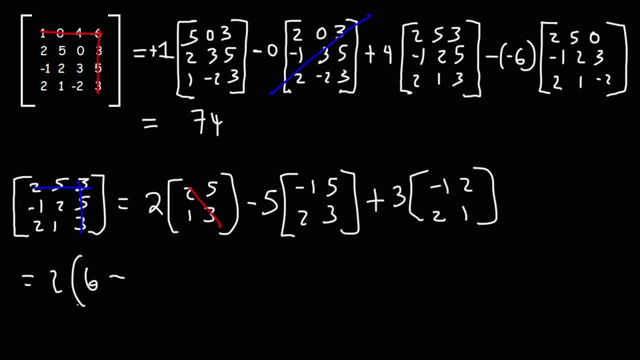 So we're going to have 2 times 3, which is 6, minus 1 times 5, which is 5. 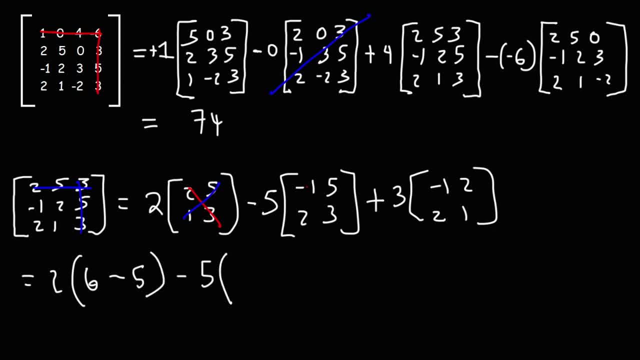 And then it's going to be minus 5. And then we have negative 1 times 3. That is negative 3. Minus 2 times 5, which is positive 10. 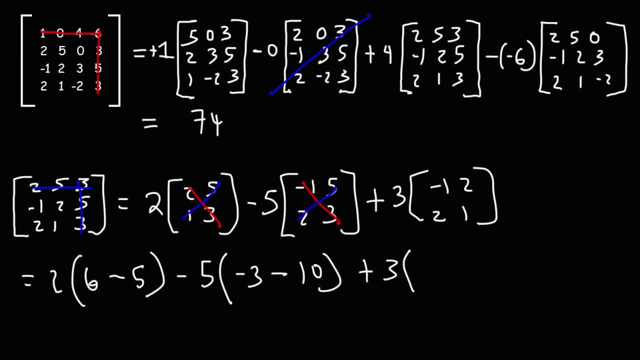 And the next, negative 1 times 1 is negative 1. And then minus 2 times 2, which is 4. 6 minus 5 is 1. Negative 3 minus 10 is negative 13. Negative 1 minus 4 is negative 5. 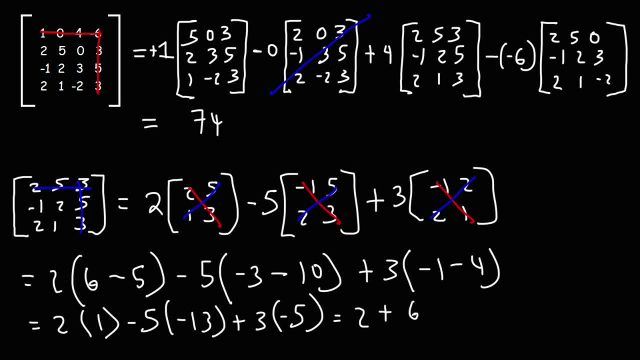 Negative 5 times negative 13. That's positive 65. 3 times negative 5 is negative 15. 65 minus 15 is 50. And 2 plus 50 is 52. 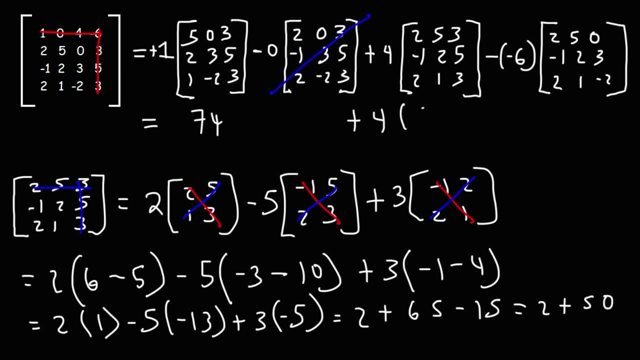 So this is plus 4 times 52. Don't forget the 4 here. And let's put a 0 for this particular 3x3 matrix. Now, let's work on the last one. 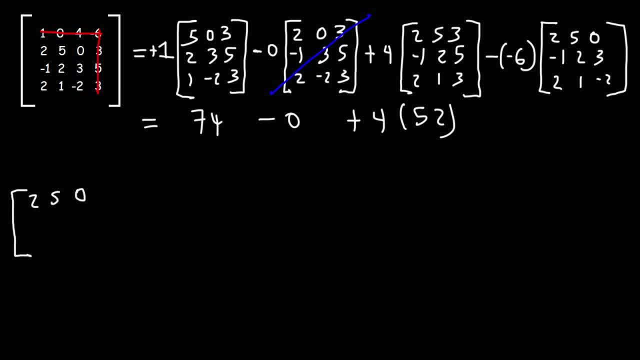 So the numbers are 2, 5, 0, negative 1, 2, 3, 2, 1, negative 2. So starting with the first number, 2, if we eliminate the first row and the first column, we're left with 2, 3, 1, negative 2. And then minus 5, eliminating row 1, column 2. We're left with negative 1, 3, 2, negative 2. 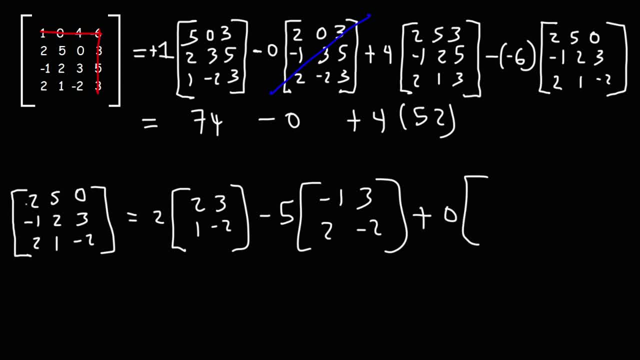 And then plus 0. And we're left with negative 1, 2, 2, 1. 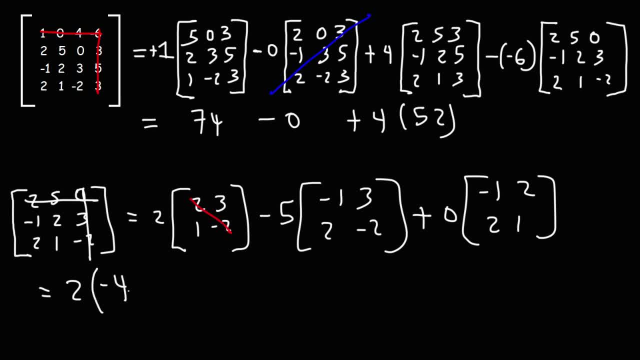 So now if we multiply 2 by negative 2, that's negative 4. Minus 1 times 3, which is 3. And then minus 5. 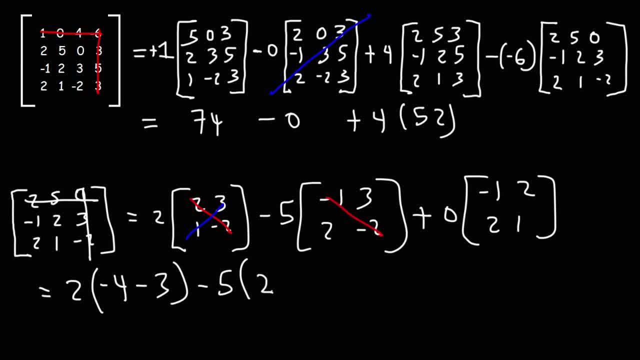 Next, we have negative 1 times negative 2, which is 2, minus 2 times 3, and that's 6. And of course, this is 0, so we can get rid of that. Negative 4 minus 3 is negative 7. 2 minus 6 is negative 4. 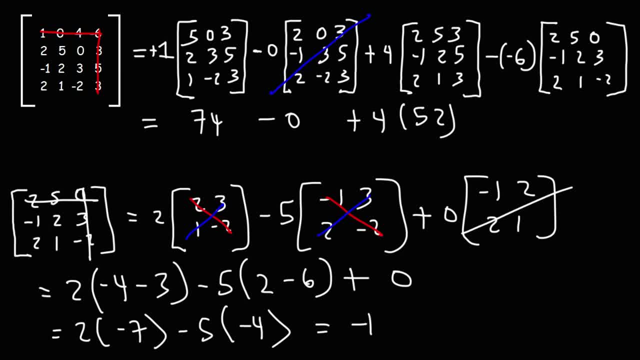 And then we have 2 times negative 7, which is negative 14. 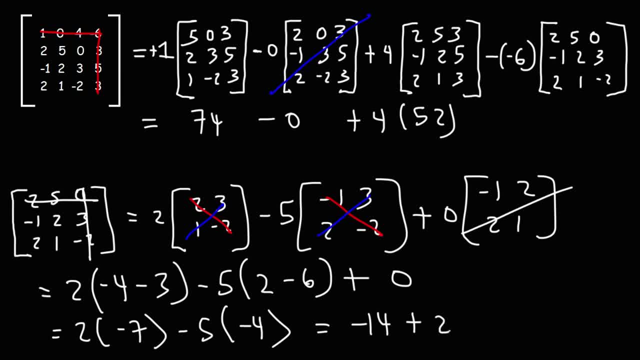 Negative 5 times negative 4, that's 20. Negative 14 plus 20, or 20 minus 14, that's positive 6. Now we also have a positive 6 out in the front. 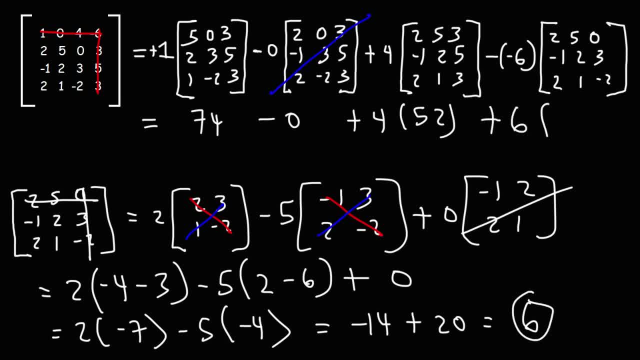 So it's plus 6 times the determinant of this matrix, which is 6 as well. So this is what we now have. 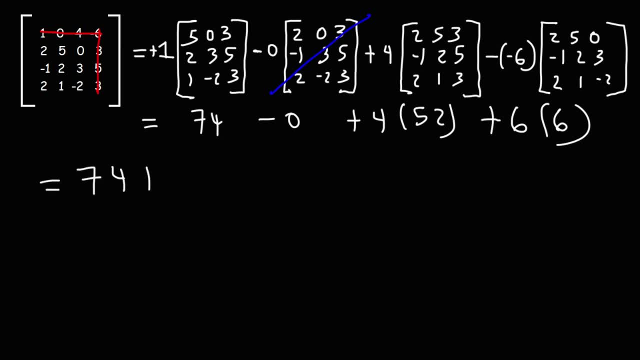 Now let's add it up together. So we have 74 plus, now 4 times 52. 4 times 50 is 2. 4 times 2 is 8. So that's going to be 208. And then 6 times 6 is 36. Now let's add it up the old-fashioned way. 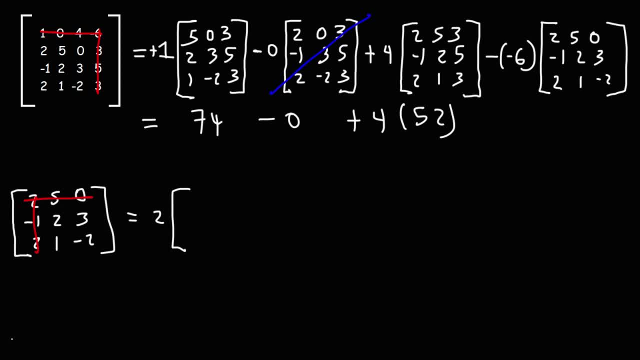 If we eliminate the first row and the first column, we're left with 2, 3, 1, negative 2.. And then minus 5, eliminating row 1, column 2. We're left with negative 1, 3, 2, negative 2.. 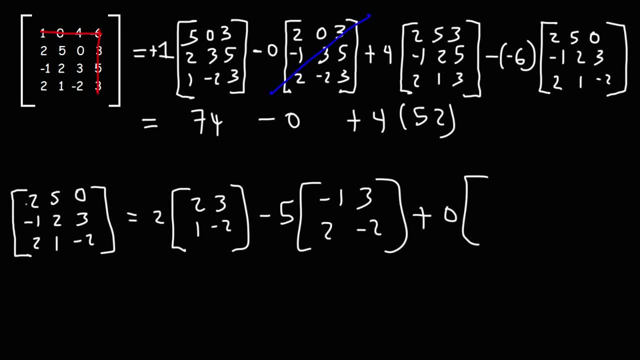 And then plus 0. And we're left with negative 1, 2, 2, 1.. So now, if we multiply 2 by negative 2, that's negative 4.. Minus 1 times 3,, which is 3.. 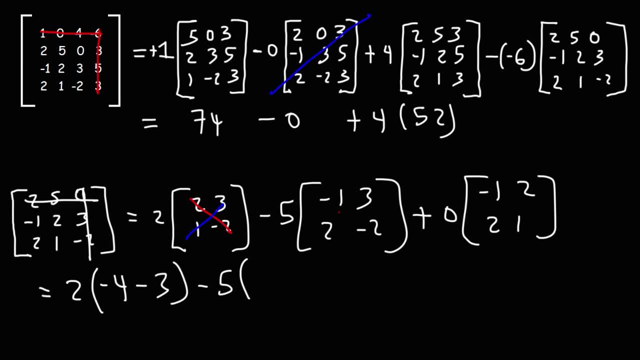 And then minus 5.. Next we have negative 1 times negative 2,, which is 2.. Minus 2 times 3,, and that's 6. And of course this is 0, so we can get rid of that. 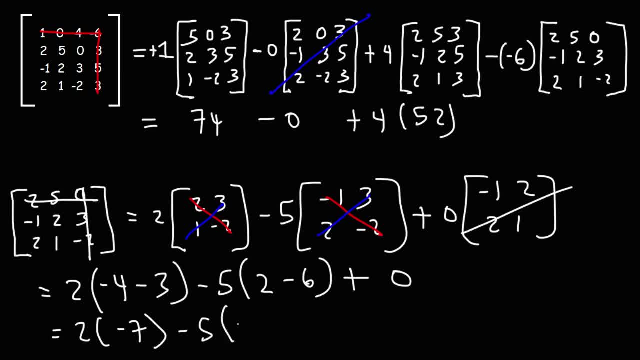 Negative: 4 minus 3 is negative 7.. 2 minus 6 is negative 4.. And then we have 2 times negative 7,, which is negative 14.. Negative 5 times negative 4, that's 20.. 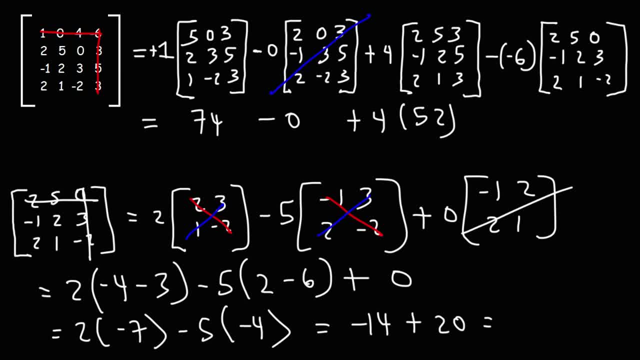 Negative: 14 plus 4.. Negative 4 times negative 4, that's 20.. Negative: 14 plus 4.. Negative 4 minus 20, or 20 minus 14, that's positive 6.. Now we also have a positive 6 out in the front. 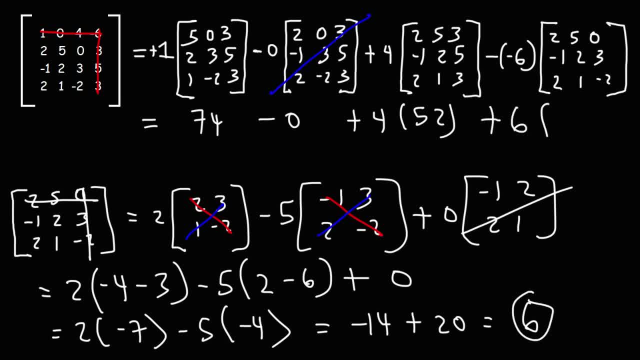 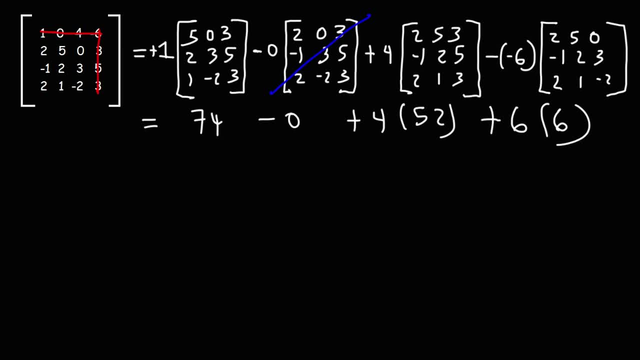 So it's plus 6 times the determinant of this matrix, which is 6 as well. So this is what we now have. Now let's add it up together, So we have 74 plus now 4 times 52.. 4 times 50 is 200.. 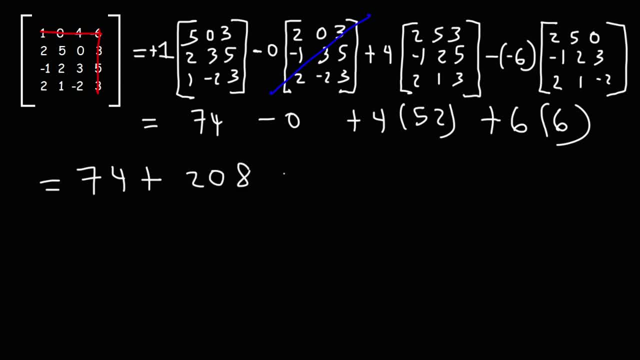 4 times 2 is 8.. So that's going to be 4.. That's going to be 208.. And then 6 times 6 is 36.. Now let's add it up the old-fashioned way: 4 and 6 is 10 plus 8, that's 18.. 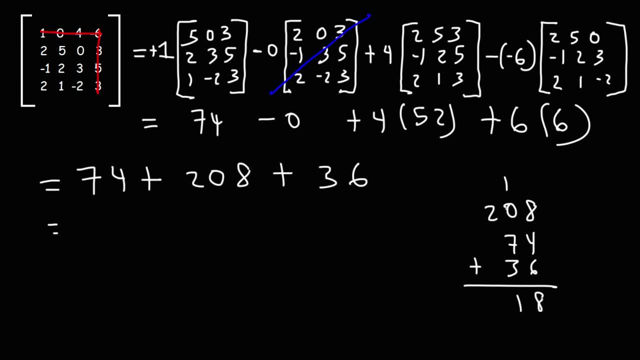 Carry over the 1.. 7 and 3 is 10 plus 1, that's 11.. Carry over the other one, 2 and 1, is 3.. So the determinant of this 3 by 3 matrix is 318.. 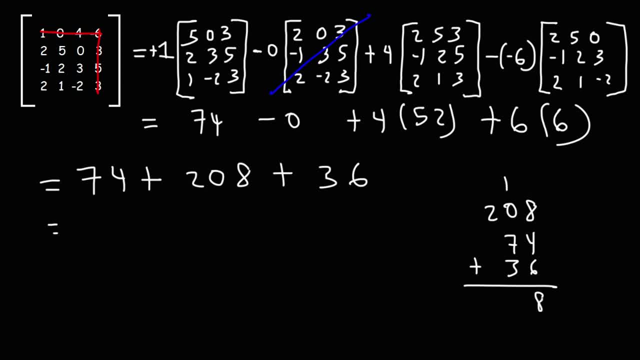 4 and 6 is 10 plus 8, that's 18. Carry over the 1. 7 and 3 is 10 plus 1, that's 11. Carry over the other one. 2 and 1 is 3. 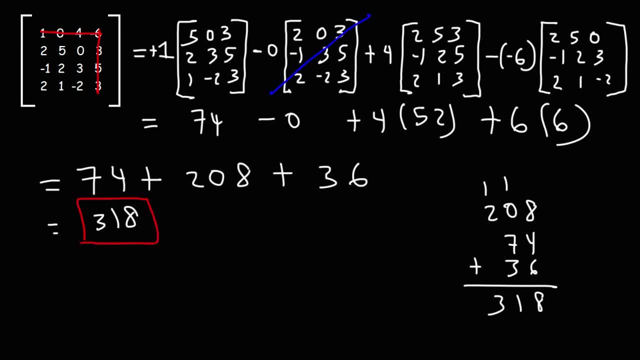 So the determinant of this 3 by 3 matrix is 318. That is the answer. 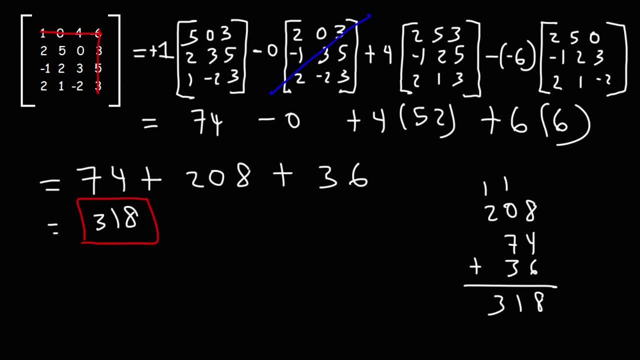 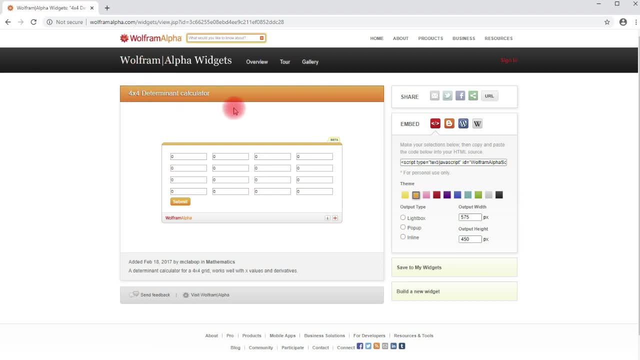 Now we can also check our work using Wolfram Alpha. So if you type in Wolfram Alpha 4 by 4 determinant calculator in Google, this page should come up. 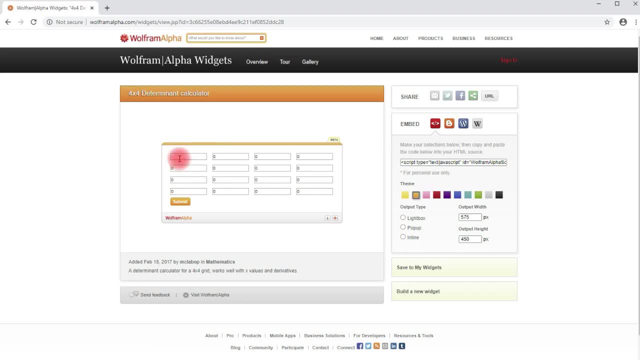 So all we're going to do is plug in the numbers in our 4 by 4 matrix. So it was 1, 0, 4, negative 6, 2, 5, 0, 3, and then negative 1, 2, 3, 5, 2, 1, minus 2, 3. And then just hit submit. And let's, there it is. 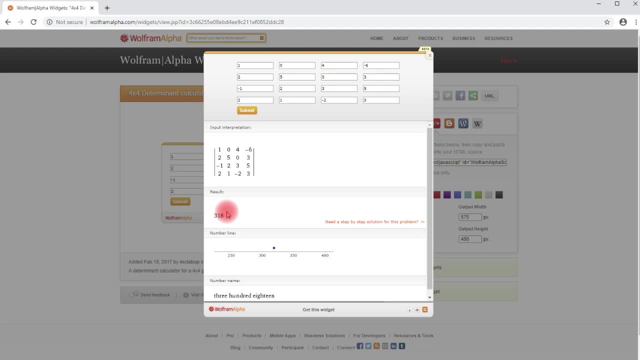 So you can see the determinant is 318. So that's a quick way to check your work to make sure that you have it right. Because after doing all that work, you want to make sure that you have the right answer. So that's it for this video. Hopefully you found it to be helpful. Thanks for watching.